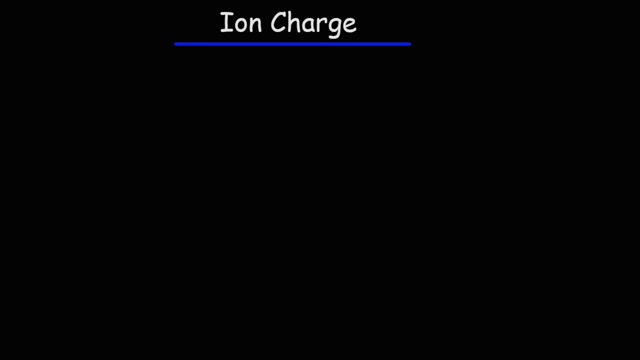 In this lesson we're going to talk about how to determine the charge of an element when it becomes an ion. So the first thing you need to be familiar with is the monoatomic ions based on a periodic table. So if you go to Google Images and if you download a periodic table, 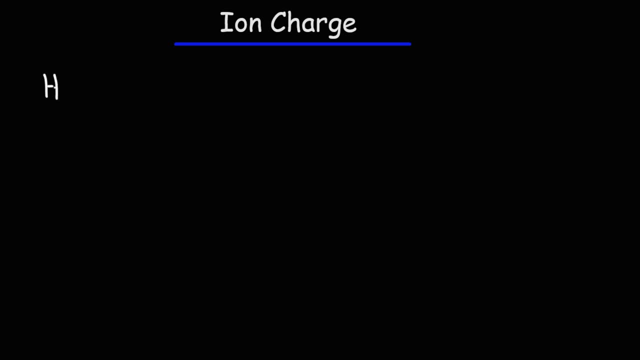 you'll see these elements on the left. You have hydrogen. After that is lithium, sodium, potassium, rubidium As a pure element. these elements have a neutral charge, But when they become an ion they will acquire a positive charge. So this is the alkali metals, Now hydrogen. 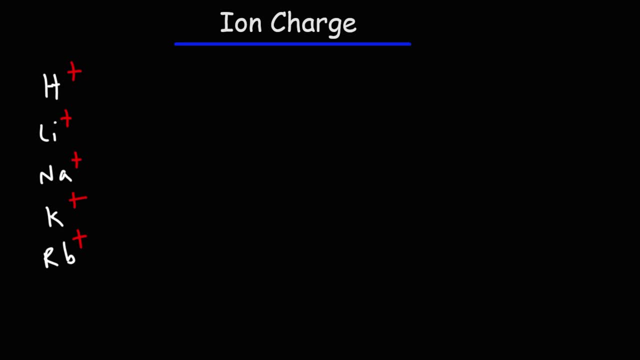 is not going to be an ion, It's going to be a positive charge. So this is the alkali metals. Now, hydrogen is not going to be an ion, It's going to be a positive charge. So this is the metal. But lithium, sodium, potassium, rubidium, those are metals. So group 1A represents the 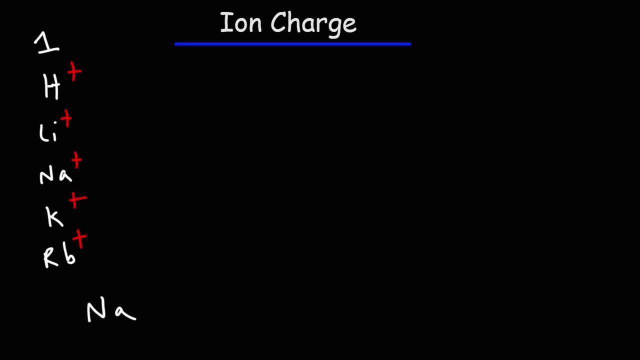 alkali metals. So, for instance, sodium has 11 electrons but only one electron in its outermost shell, So it only has one valence electron. When sodium reacts and gives up that valence electron, it becomes an ion. So the number of valence electrons that an atom has can give you a good idea of what kind of charge. 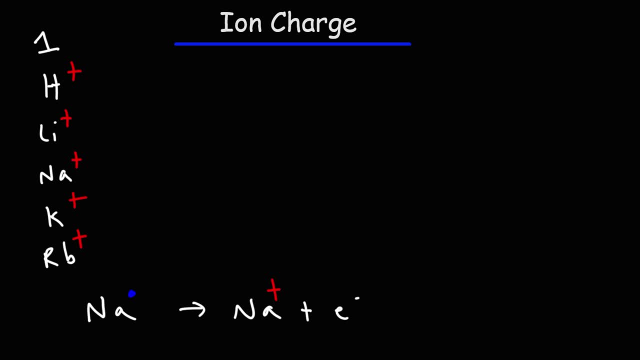 it's going to have when it becomes an ion. So elements that typically have one valence, electron, will usually form ions with a plus one charge. Now in group 2, we have the alkaline earth metals, So like elements like beryllium, magnesium and copper. So these are the elements that are going 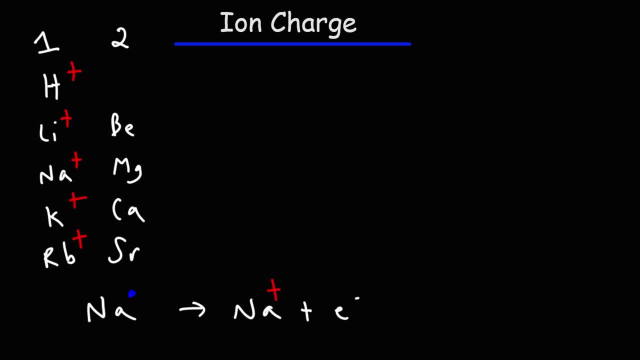 to be a positive charge. So, for instance, calcium, magnesium, calcium, strontium, These elements are in group 2 and they have two valence electrons. So because they have two valence electrons to give up as an ion, they will typically form a two-plus charge. So calcium, which has two valence electrons. 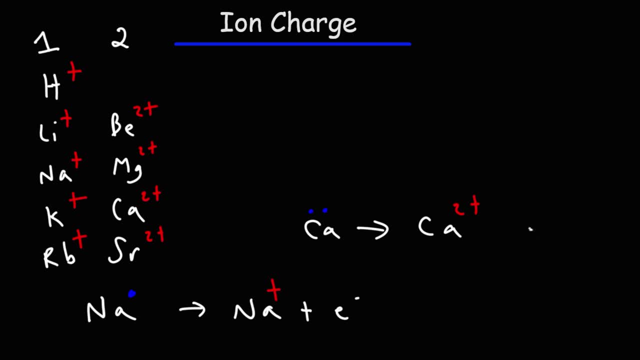 those two electrons forming the calcium, two plus ion. So metals, they typically form positively charged ions, whereas nonmetals they typically form negatively charged ions. Now in the middle we have the transition metals, which we could talk about that later in this video. 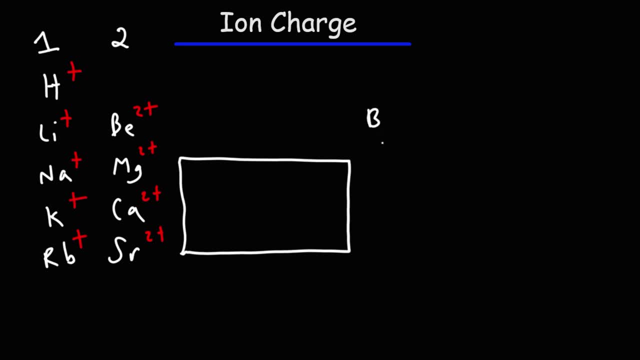 But to the right we have elements like boron, aluminum, gallium, indium, thallium, So that's the group 3A elements also known as group 13.. Group 14, or group 4A, we have carbon. 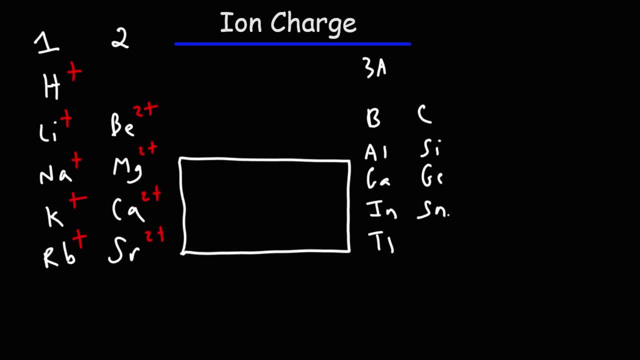 silicon, germanium, tin and lead. Now this group. they have three valence electrons, So you might be thinking that they will form a three plus charge, which in fact they do, But some of these elements also form a plus one charge. 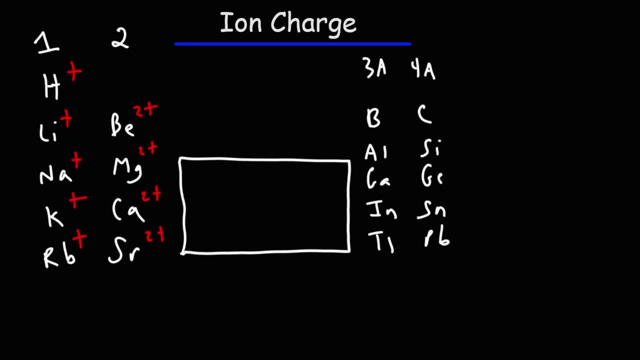 Now I don't know for you, the viewer, if you've learned electron configuration, but if you have these elements here, they have S electrons. these elements here, they have P electrons. So for indium actually let's use aluminum. 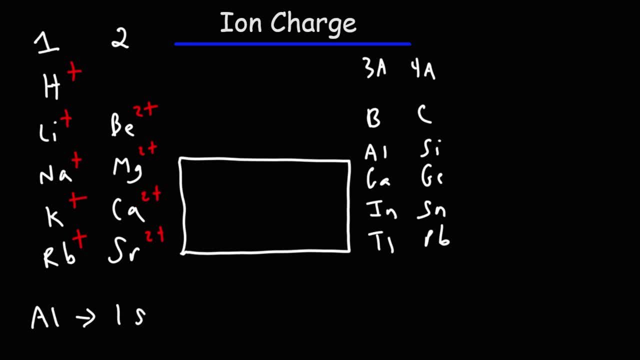 Aluminum. when you write the electron configuration, it's 1s2, 2s2, 2p6, 3s2, 3p1.. Notice that it has three valence electrons. When aluminum gives up those three valence electrons, 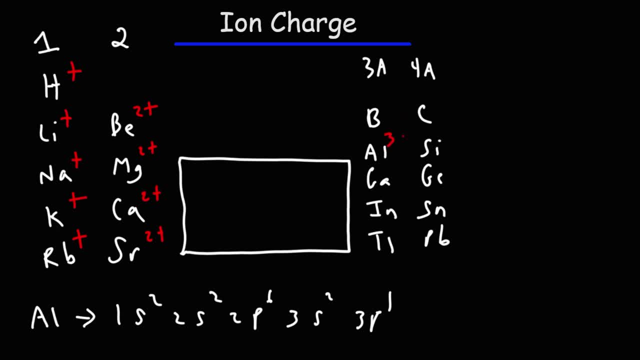 it will have a three plus charge. Now, the elements below that, like gallium and indium and thallium, instead of giving up all three electrons, sometimes they could just give up one electron, And so they can have a plus one charge. 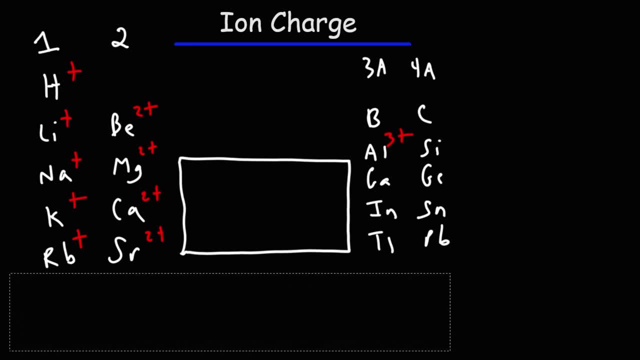 So understanding electron configuration will help you to get a better understanding of what type of charges certain ions or certain elements form when they become ions. So gallium, indium, thallium, they will typically form a plus one or a plus three charge. 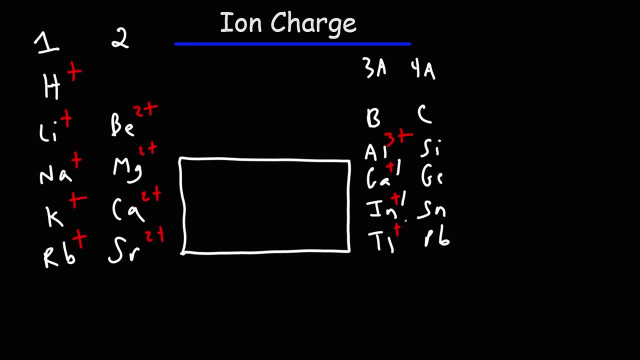 But you can also form a four plus charge Depending on the reaction conditions. Now here we have group 4a elements, which has four valence electrons, and they can form a four plus charge, But, like these elements, some of them can have a two plus as well. 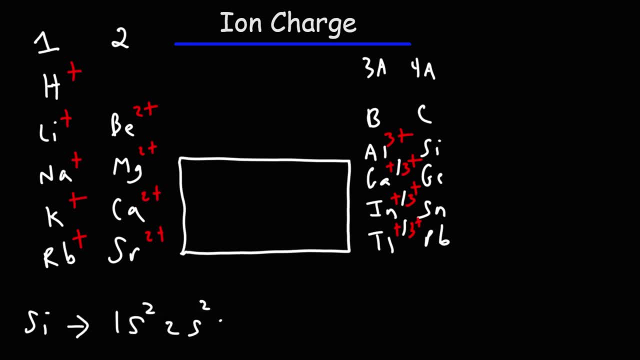 configuration of silicon. It's 1s2, 2s2, 2p6, 3s2, 3p2.. Now if silicon gives up all four of its valence electrons, it's going to have the 4 plus charge. If it gives up only two. 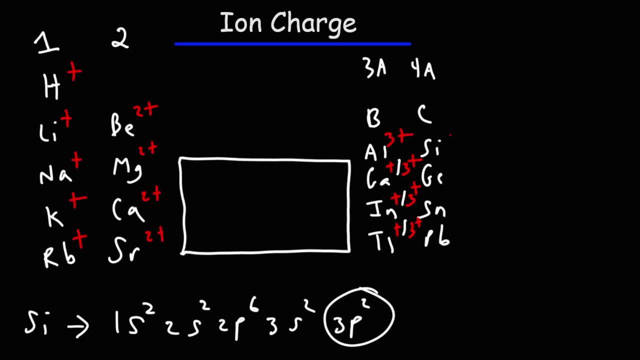 it's going to have the 2 plus charge. So silicon, germanium, tin and lead, when you research them, you'll find that they can have the plus 2 oxidation state or the plus 4 oxidation state. Now group 5a, elements like nitrogen, phosphorus, arsenic. 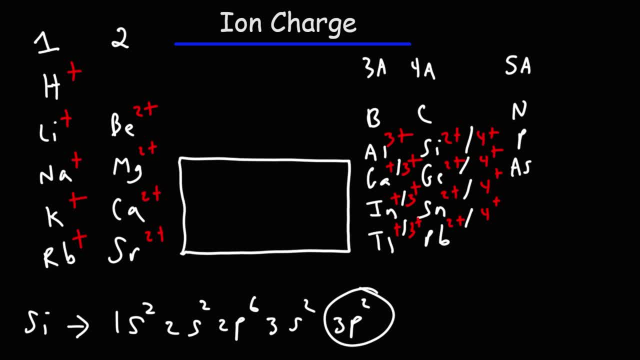 these are nonmetals. Arsenic may be considered a metalloid- It's kind of close to that region- But nitrogen and phosphorus are nonmetals. Remember we said that metals like to give up electrons to form positively charged ions known as cations, Nonmetals, which is typically 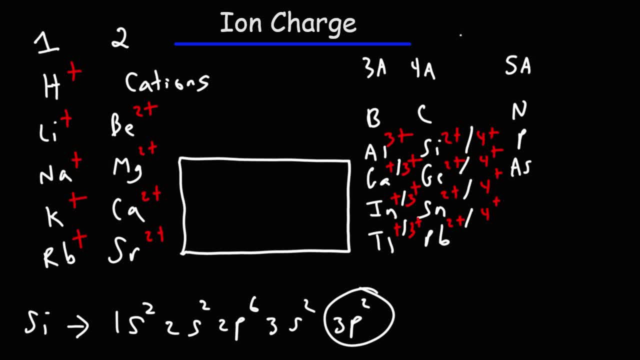 in this side of the periodic table. they like to acquire electrons and form negatively charged ions called anions. Now, nitrogen has five valence electrons And it wants to acquire electrons to have a field octet, So it wants to gain three electrons. 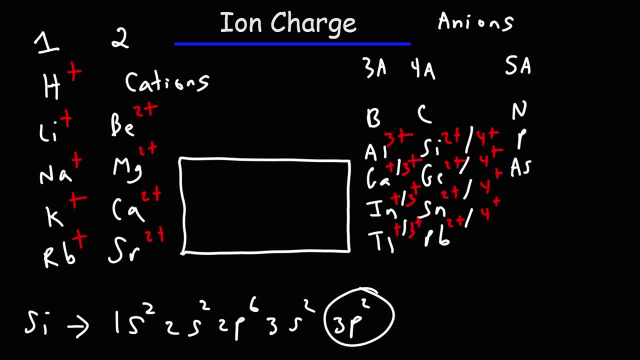 to satisfy its octet requirement. Once it gains those three electrons, it's going to have a 3 minus charge. So group 5a elements: they will typically form a 3 minus charge. Now group 6a elements: they have six valence electrons. This is like oxygen, sulfur, selenium And they only need 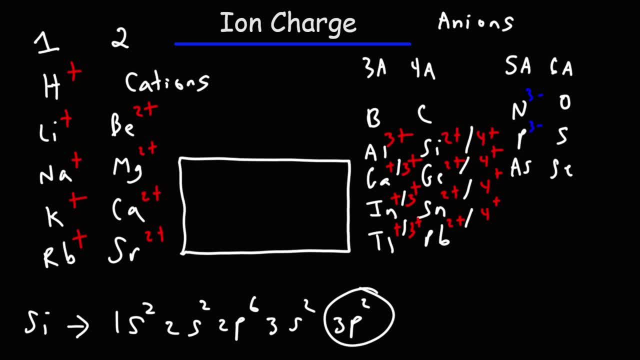 two more electrons to form a 3 minus charge. So group 6a elements. they have six valence electrons. They only need two more to get to 8. Once they acquire those two electrons they will have a charge of 2 minus. And then you have the group 7a elements like fluorine, chlorine bromine. 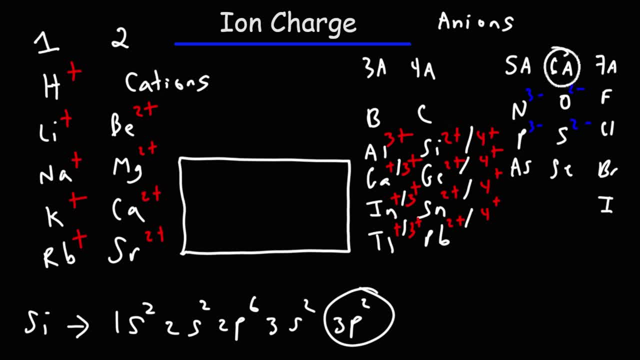 iodine. These are the halogens, Group 6a. they're the chalcogens, Now the halogens. they have seven valence electrons. They only need one more to get to 8. So they will generate a negative one charge once they get that one electron to have eight electrons. 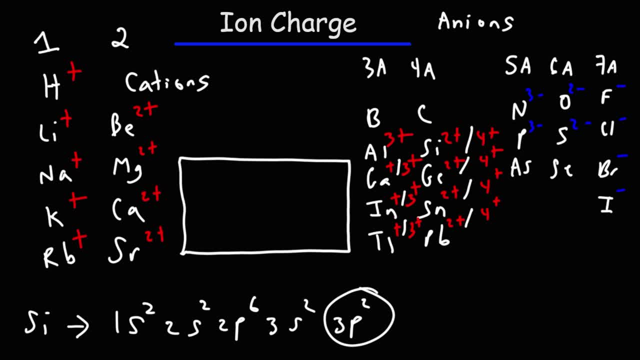 in their outermost energy level. So that's how you could determine the charge of an element when it becomes an ion using a periodic table. It has to do with the number of valence electrons. When metals give up their valence electrons, they will acquire a positive charge, And that positive charge is 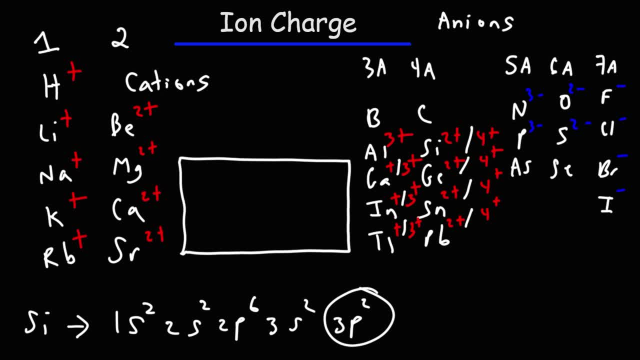 determined by how much of the valence electrons they have. So that's how you could determine the charge of an element when it becomes an ion, using a periodic table. The nonmetals, when they acquire electrons, the number of electrons that they acquire will determine the. 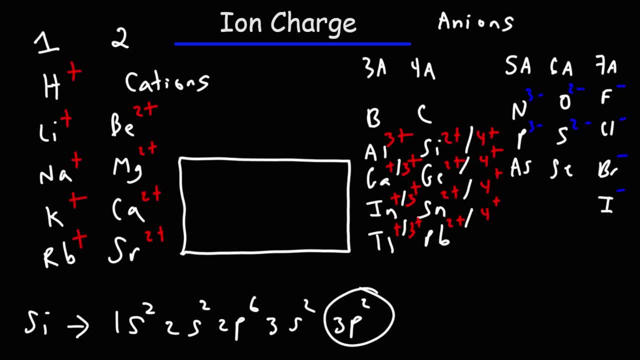 charge that they're going to have. So here's a formula that will help you to calculate ion charge. The ion charge is the difference between the number of protons that an atom has and the number of electrons. So let's use aluminum as an example. Aluminum, if you look up in a periodic table. 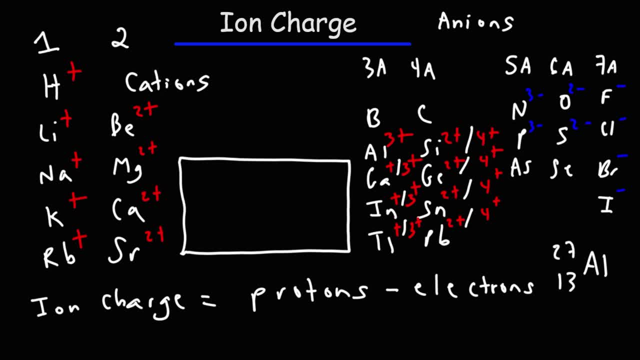 it has a mass number of 27 and an atomic number of 13.. Now an atom has an equal number of protons and electrons, So atoms are electrically neutral Ions. the reason why they have a charge is because the number of protons and electrons are different. 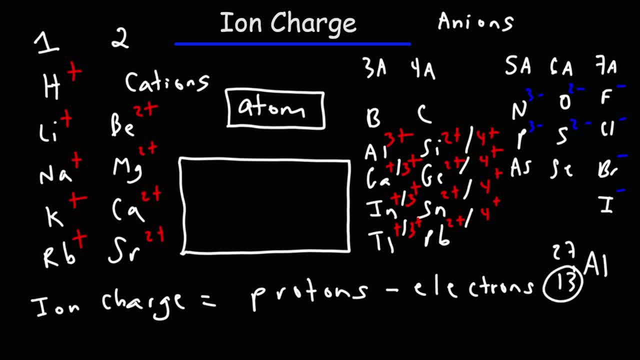 And another thing you need to know is that the atomic number of an element is equal to the number of protons, So aluminum will always have 13 protons. If that number is different, it's no longer aluminum As an atom. aluminum will have 13 electrons, And so its ion charge will be zero. 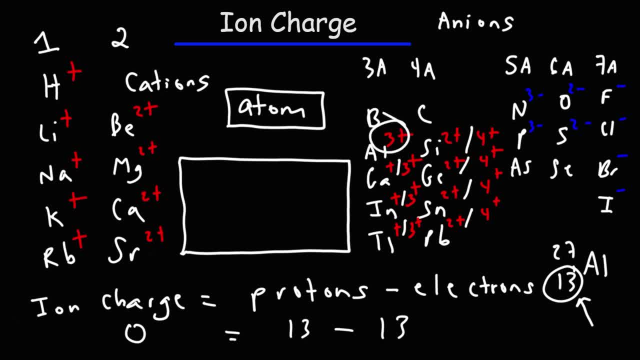 Now, in order to form this 3 plus charge, aluminum has to give up 3 electrons. When it does that, it will have 10 electrons, And so 13 protons minus 10 electrons. you get a charge of plus 3 or 3 plus. 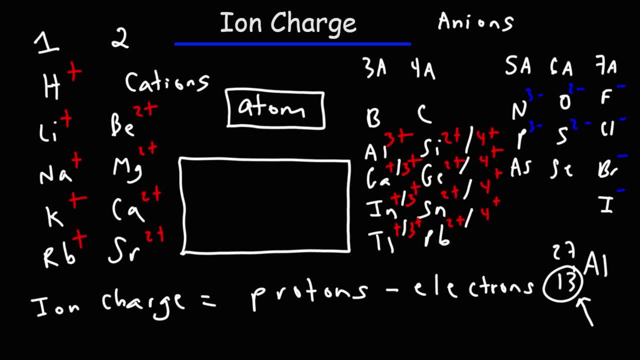 In the case of oxygen, oxygen has a mass number of 16 and an atomic number of 8.. So, as an atom, oxygen has 8 protons, 8 electrons, so its ion charge is zero. Now when oxygen gains 2 more electrons to satisfy its octet requirement, it will have 10 electrons. 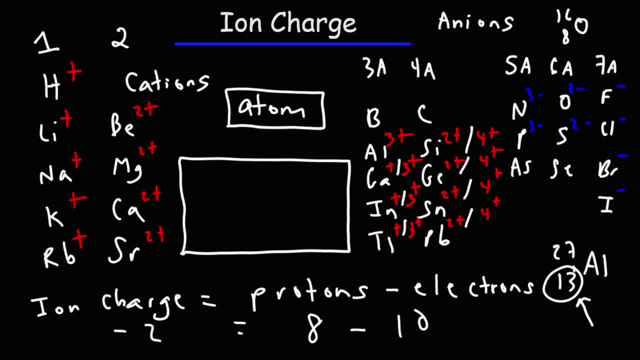 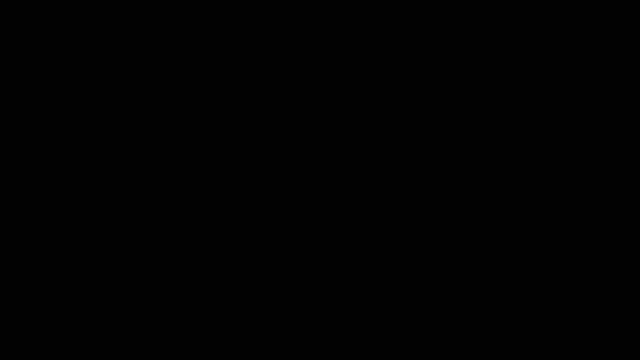 And so at that point its charge will be negative 2.. So that's the formula for calculating ion charge. It's simply the difference between the number of protons and electrons that the ion has. Now, sometimes you might be given the formula of an ionic compound. 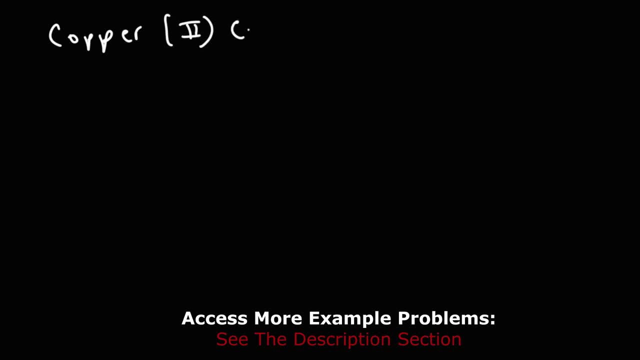 Let's say it like this: copper to chloride. When you see this Roman numeral, it tells you the oxidation state of the metal. So it tells you that you're dealing with the copper ion, Because when you're dealing with transition metals, many of the transition metals have multiple oxidation states. 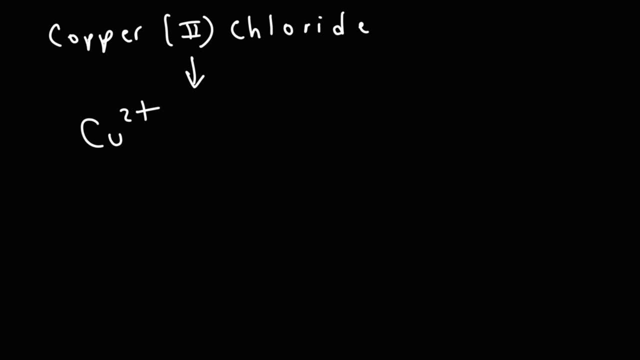 So as an ion they can have different charges. So, even like some of the non-transition metals like lead, Lead has two oxidation states. We talked about it already: 2 plus and 4 plus. So if you see a compound that says lead oxide, 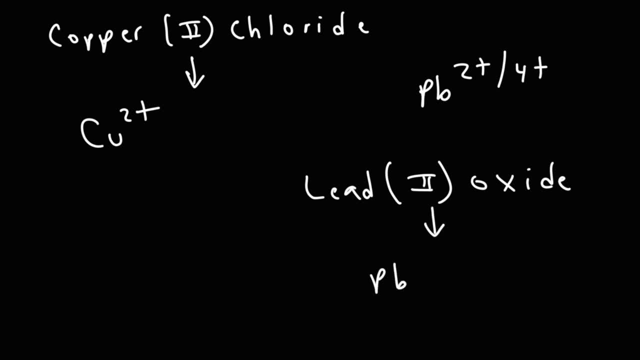 the Roman numeral 2 tells you you're dealing with Pb2+. If you see a compound that says lead sulfide, well, in this case lead has a 4 plus charge. So make sure you understand that difference. But with that being said, let's go over some of the common charges of the common transition metals that you'll deal with in a typical chemistry course. 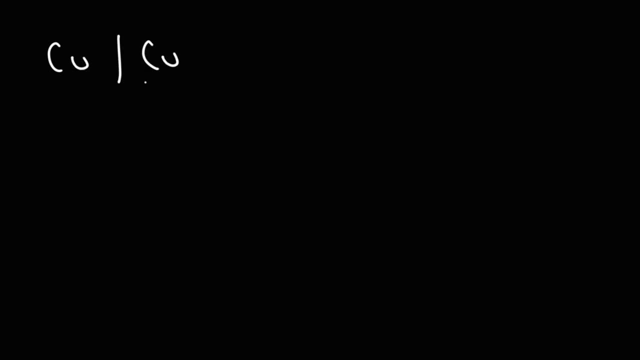 So the most two common oxidation states for copper are these two: The copper plus charge and the copper 2 plus ion. Now the copper 2 plus ion is more common than the copper plus 1 ion. So if you don't have a compound with a Roman numeral and if you have to guess, 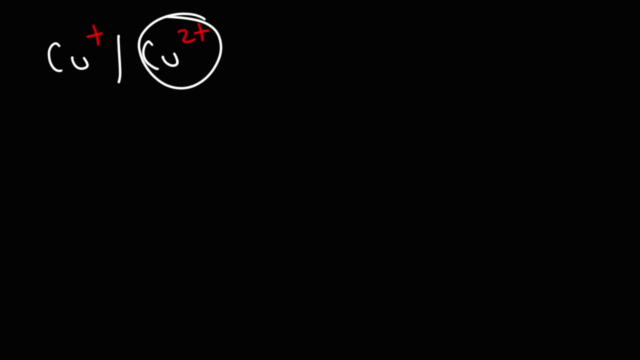 chances are, it's more likely to be copper 2 plus than copper plus 1.. But both of these can occur. Now for iron metal, there's two common oxidation states: 2 and 3. So those are the two most common ions you'll see with iron metal. 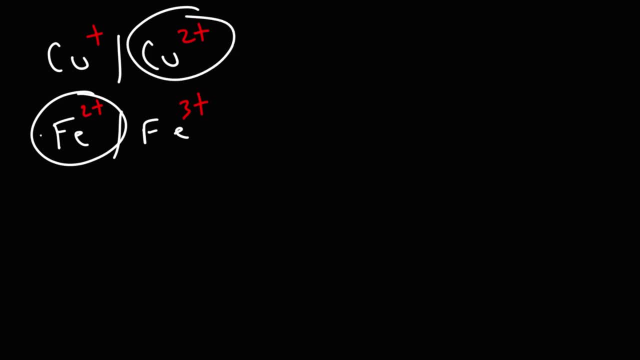 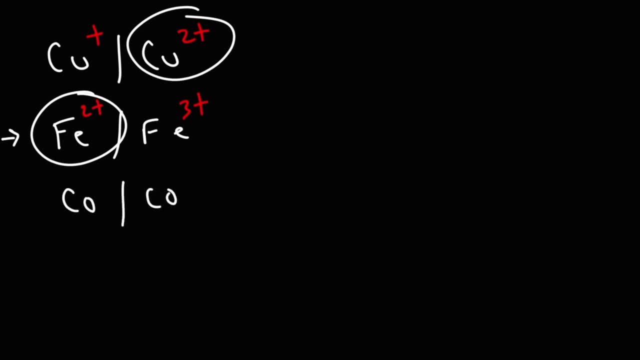 So iron is usually most likely to be more stable than Fe3 plus, So iron is usually most likely to be more stable than Fe3 plus. Now, cobalt has two common oxidation states. It has others too, but these are the most common. 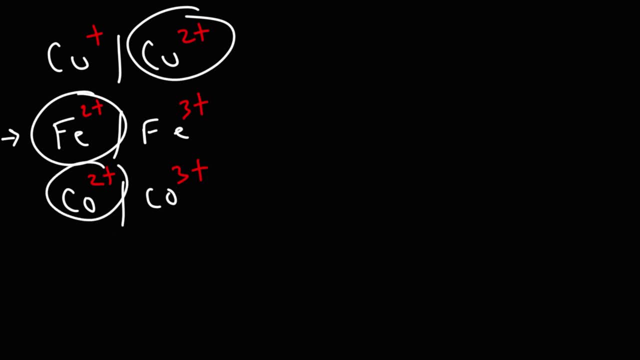 The 2 plus and the 3 plus ion. The 2 plus ion is more stable, so that's going to be more common: Zinc, Nickel, Cadmium. most of the time they will have the 2 plus oxidation state. Now, this is not always the case. 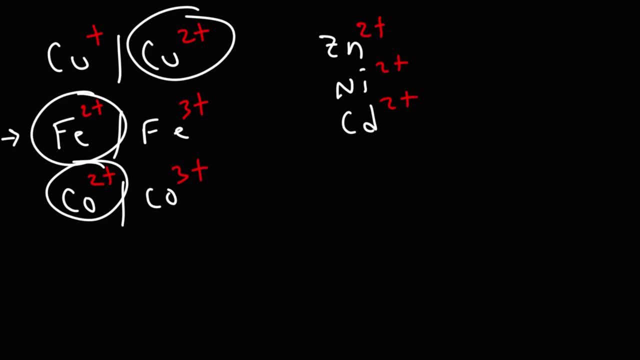 but in a typical general chemistry course, more than 90% of the time those will be the charges of those ions. For chromium it's usually one of these two forms, 2 plus or 3 plus. 99% of the time silver is in the plus one oxidation. 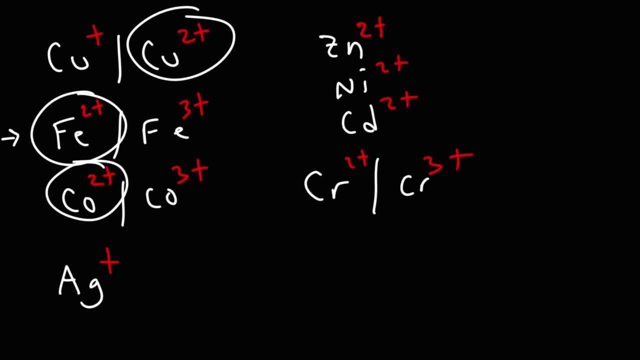 state. I've also seen a plus three oxidation state for other compounds, but more than 90% of the time it will be Ag plus one Gold. I've seen plus one and plus three for this. So if you want to commit that to memory, those are some. 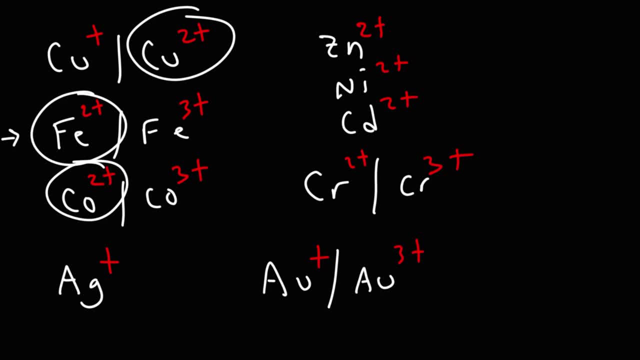 charges that those elements will form as an ion. Now for the polyatomic ions. for the most part, you need to commit this to memory. What I'm going to do is I'm going to post some videos in the description section below this video, one of which will be the polyatomic ions that you need to know. so feel free to. 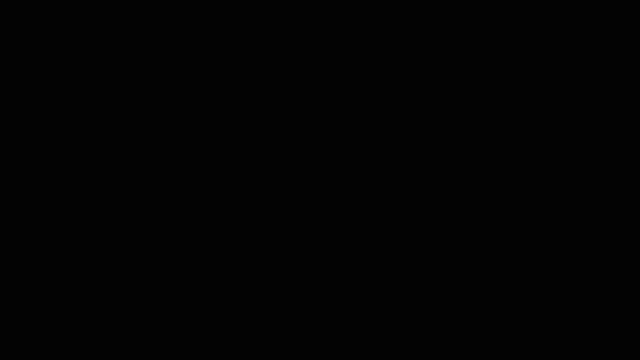 watch those videos if you want to memorize the charges of these ions. So sulfide, which we talked about earlier, this is what is known as a monoatomic ion. Mono means one, poly means many, Sulfate, SO3, two minus. that's a polyatomic ion, because this ion is 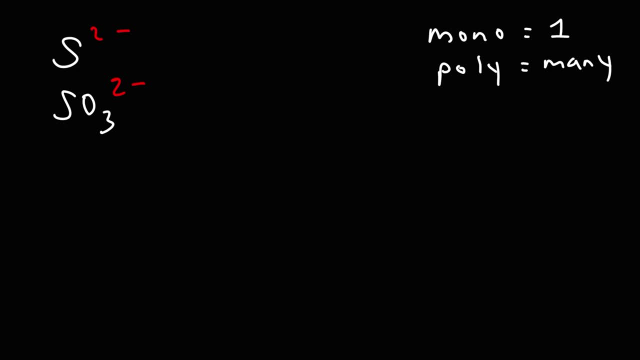 composed of many atoms: one sulfur atom and three oxygen atoms. Sulfate, that's also a polyatomic ion. Notice that the sulfur ions- they typically have a two minus charge. You, The monatomic ion, phosphide, has a 3- charge. Phosphite and phosphate also have a 3- charge. 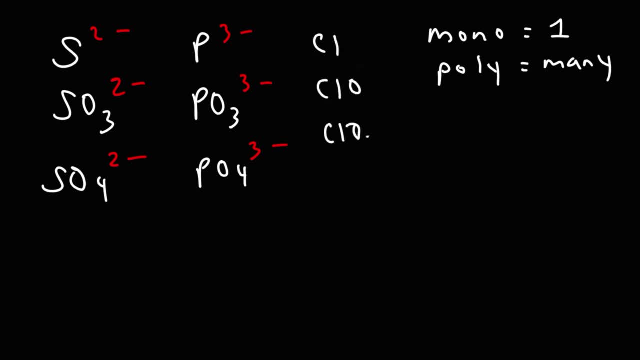 Now this works for the halogens as well. So chloride bromide iodide, they follow this trend. Chloride has a negative 1 charge, and the same is true for hypochlorite, chlorite chlorate and perchlorate. 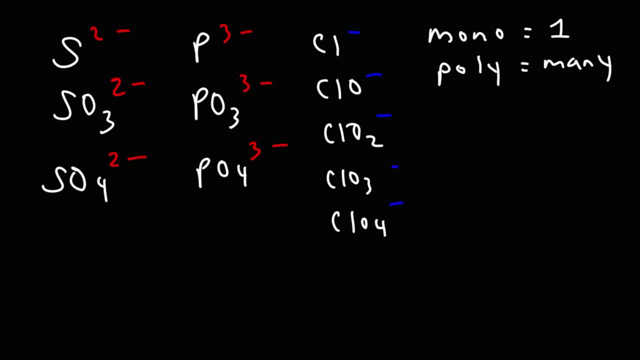 They all have the same charge, So at least that'll help you if you're trying to memorize this Now. not all elements follow this trend. Nitride has a 3- charge, but nitrite and nitrate has a negative 1 charge. 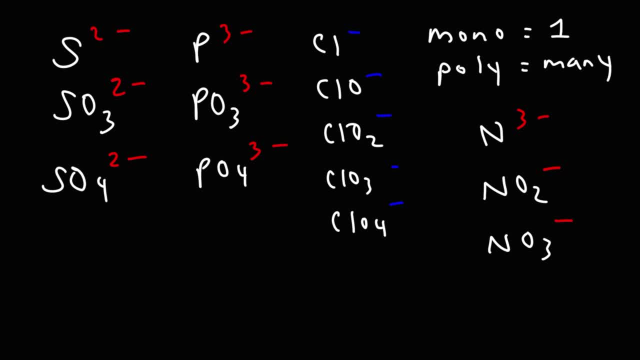 So for those elements it's different. And for other polyatomic elements you just have to commit them to memory. So like cyanide, ammonium carbonate, Acetate, most of these you have to commit to memory. Now there's something else that can help you to determine the charge of an ion. 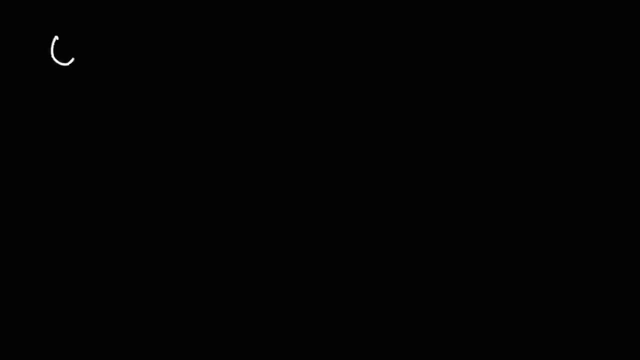 particularly if hydrogen is evolved. So, for instance, oxide has a negative 2 charge And let's say we want to determine the charge on hydroxide Whenever you add a hydrogen to a negatively charged ion and you combine them together to form a new ion. 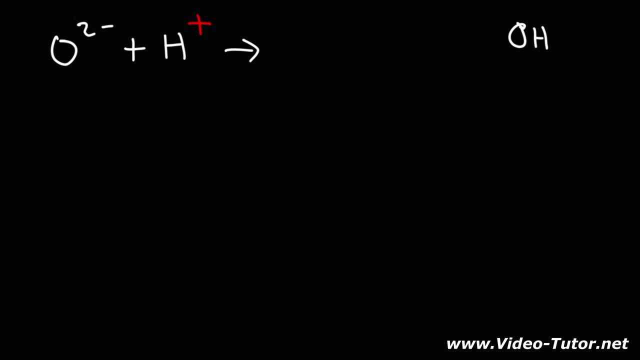 these ions. they're attracted to each other because they have opposite charges. Opposites attract like charges repel. When you combine these two ions, the ion of this charge will be the sum of these two exponents. So if you were to add negative 2 and positive 1, you're going to get negative 1.. 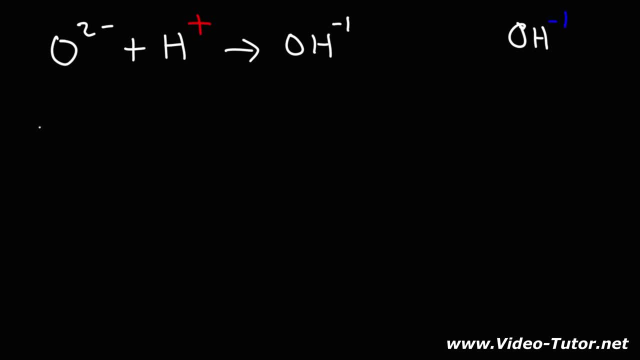 So hydroxide has a minus 1 charge. Consider this example: phosphate, which has a negative 3 charge. If you add a hydrogen ion to it and you get monohydrogen phosphate, negative 3 plus 1 will give you negative 2.. 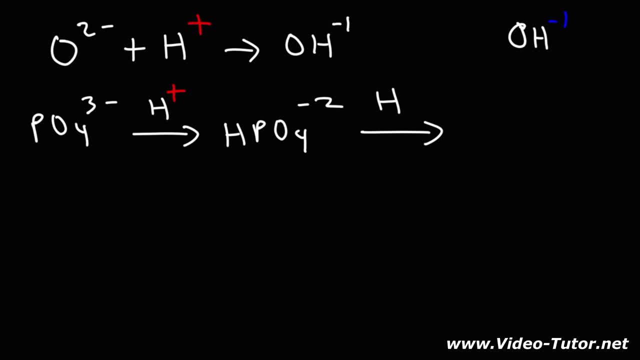 So this has a negative 2 charge. If you add another hydrogen to it, the charge is going to decrease. It's going to increase by 1.. So negative 2 plus 1, this is going to be H2PO4. now 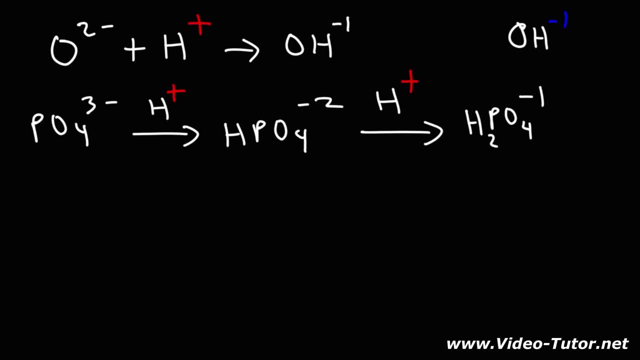 And so it's going to be minus 1, and so forth. So, for instance, let's say: if you have this substance, bisulfate or hydrogen sulfate- Actually that's bisulfite or hydrogen sulfite- What is the charge on hydrogen sulfite? 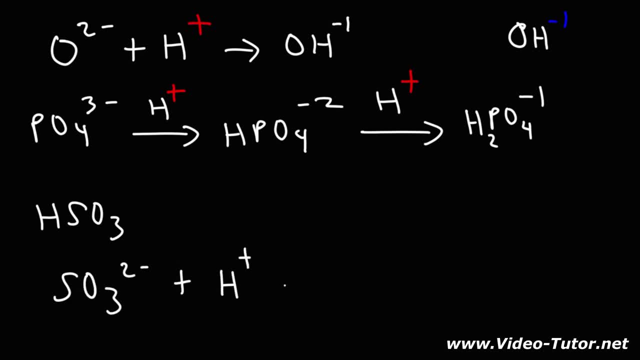 You know that sulfite has a negative 2 charge. Hydrogen has a plus 1 charge. So if you combine them together- negative 2 plus 1, that will give you a negative 1 charge. Now, earlier we said that ammonium has a plus 1 charge. 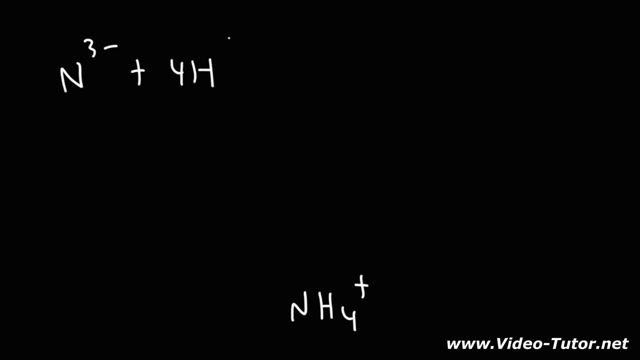 So if you were to combine nitride with 4 hydrogen ions, this will give you ammonium. So if we were to do the math, we have negative 3 and we have 4 plus 1 ions. So that's negative 3 plus 4.. 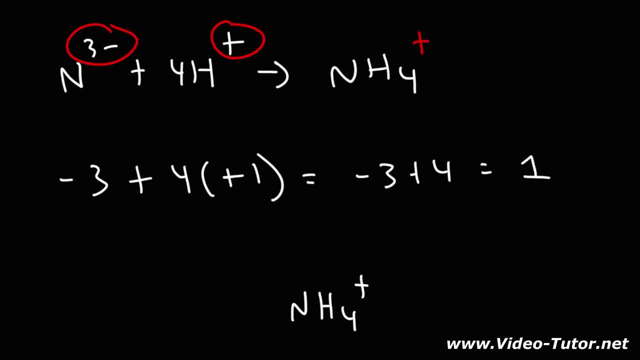 That will give us positive 1.. So ammonium has a plus 1 charge. So that's another way or another technique that you can employ to determine the charge of an ion or even polyatomic ions. But for the most part you're going to have to memorize the polyatomic ion list. 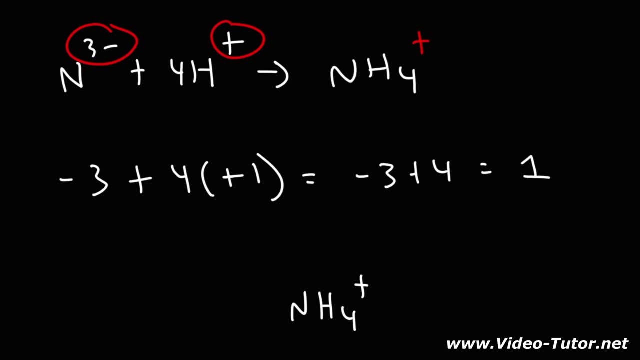 So that's it for this video. Don't forget to check the links in the description section below for other related chemistry topics, And thanks for watching.